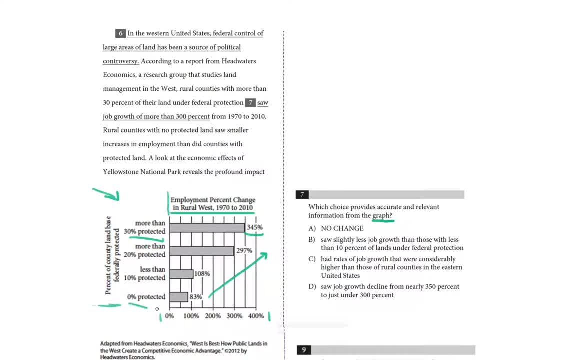 you have employment growth of 345%. If it's 0% protected, the growth still exists, but it's only 83%. So let's take a look at the question, which is just going to ask us to interpret the graph and see which choice that fits into this paragraph matches the 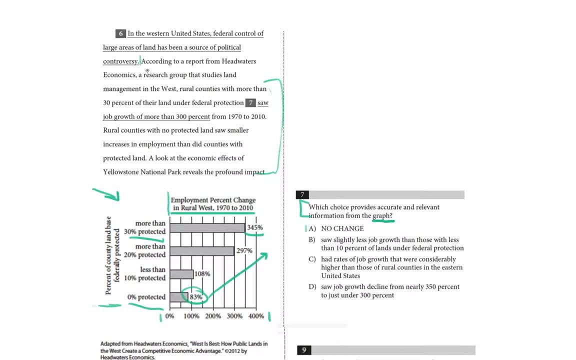 information from the graph. So let's take a look. According to a report from Headwaters Economics, a research group that studies land management in the West rural counties with more than 30% of their land under federal protection- and here's the underlying part- 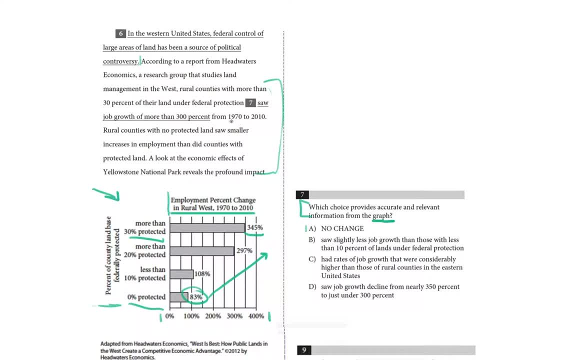 here's choice A saw job growth of more than 300% from 1970 to 2010.. Now, I think that's exactly what we saw in the graph. Hold on real quick: 300%, 30%, 30% of their land, Well, specifically, more than 30% of their land. Yeah, and that's this. 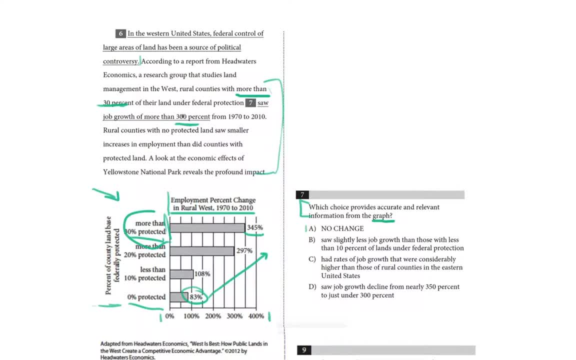 first bar graph here: 345% is more than 300.. This is the answer. Cool, Great, Honestly on test day. that's all I'd need. I feel confident about that. I'd move on, But for the purposes. 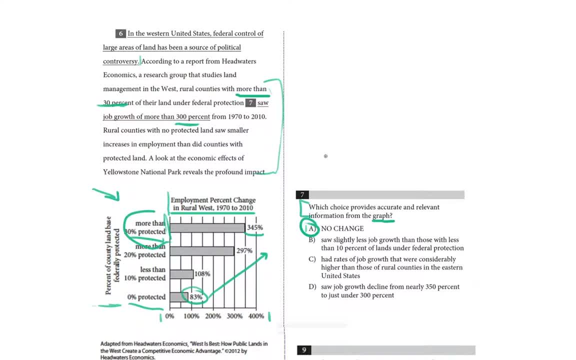 of this instructional video. let's just check them out and see. Rural counties with more than 30% of the land under federal protection saw choice B slightly less job growth than those with less than 10% of lands under federal protection. So this is showing that these two, the 108% growth and the 83% growth, are greater job. 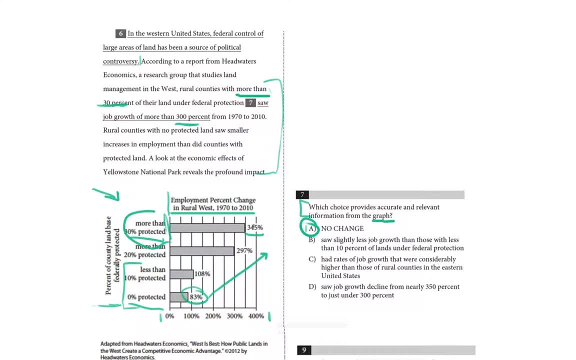 growth than the 30% that this 345 is actually smaller, less than 108 or 83. And that's not true. Choice C had rates of job growth that were considerably higher than those of rural counties in the eastern United States. That's not what this graph is about. It's about the 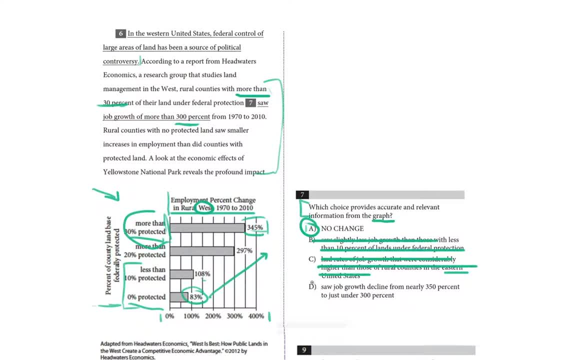 rural West, so we can't even evaluate that Choice D. the counties with more than 30% of their land under federal protection saw job growth decline from nearly 350% to just under 300%, If you were not reading the graph. 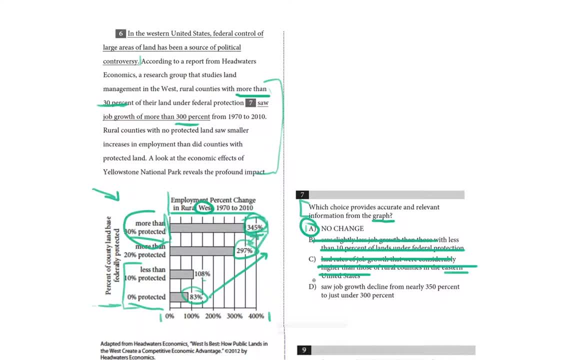 closely, it would be possible to choose D as a mistake. But we're not looking at job growth decline. This is the amount of job growth that occurs in a bunch of different counties during a specific period. All of these employment percent changes are positive.